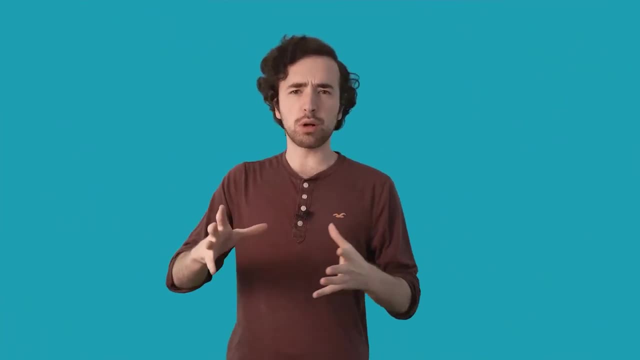 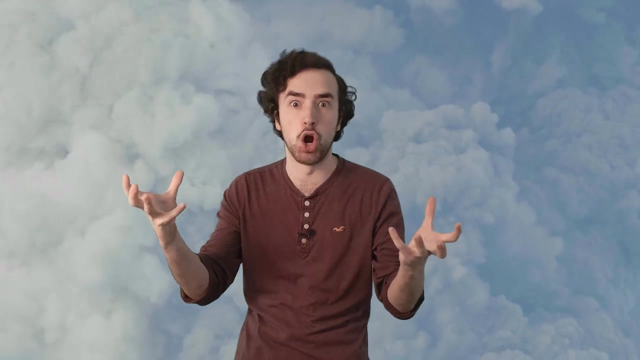 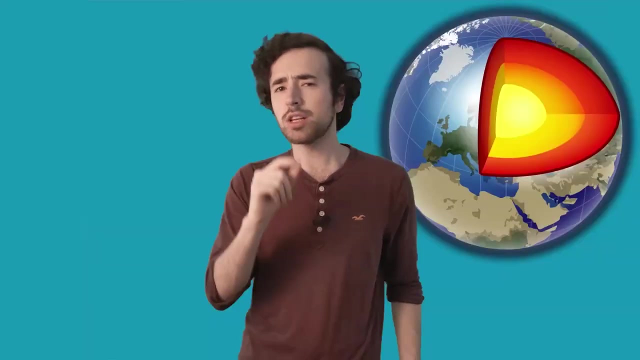 Hey everyone, it's Justin here and welcome to today's episode of Catastrophic Natural Disasters. That's right: devastating volcanoes, cataclysmic earthquakes. We'll also be taking a brief look at the Earth's layers and plate tectonics, but mostly we're talking about Catastrophic Natural. 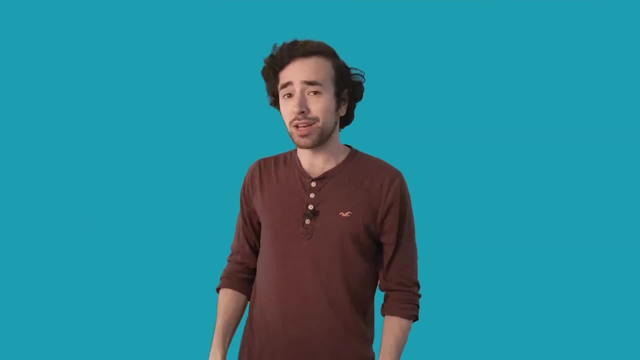 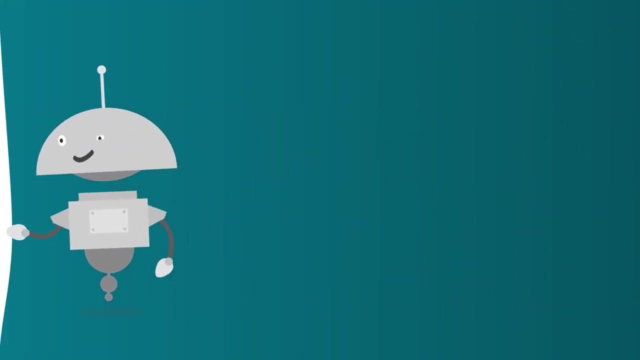 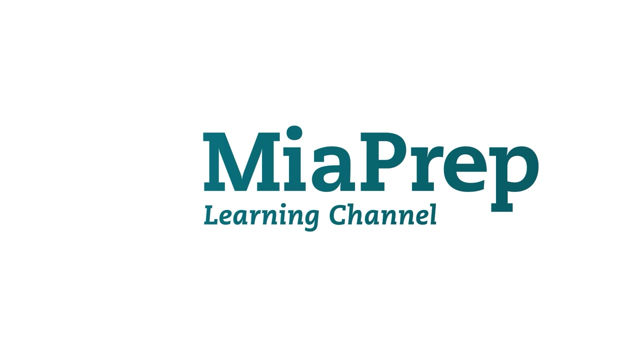 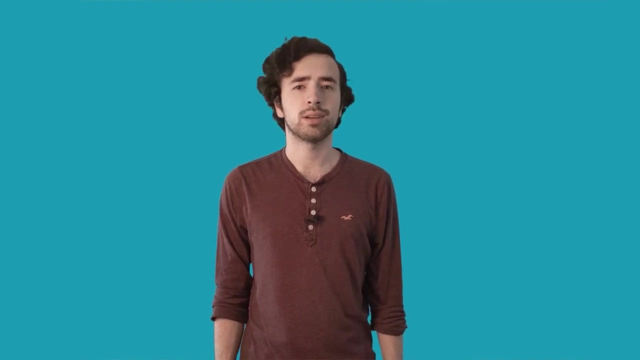 Disasters. So get your hard hats and your seismometers, because this ride can get a little bumpy. Imagine for a moment that it's the year 79 AD and you're in the ancient Roman city of Mycenae because your uncle is a military officer. 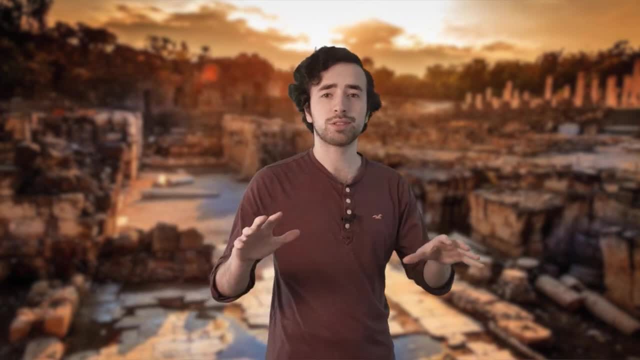 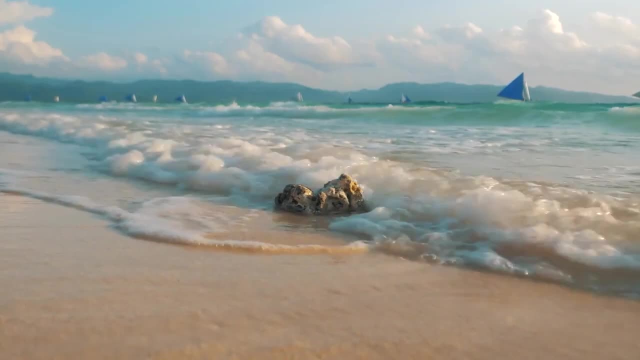 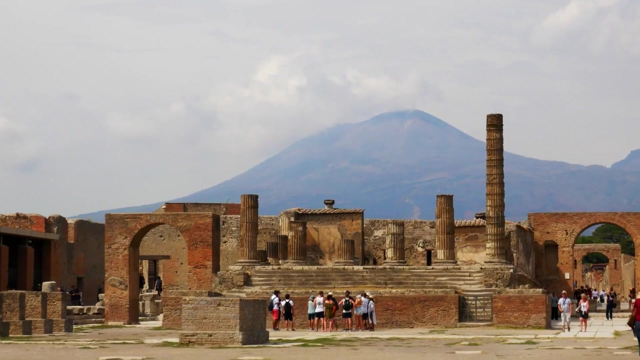 Stationed there. you're out on the terrace eating your breakfast, enjoying the magnificent view: the Bay of Naples, Mount Vesuvius, the bustling resort city of Pompeii. You are living your best life right now and you're about to shove this beautiful wheat. 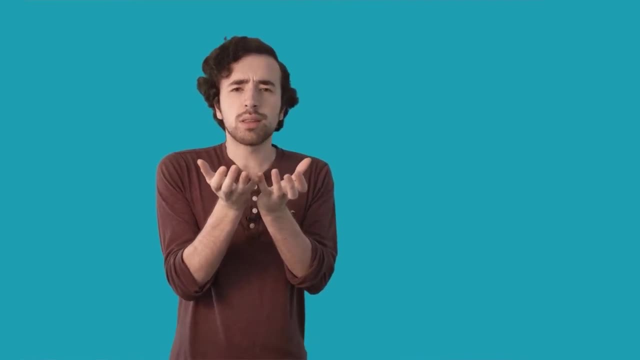 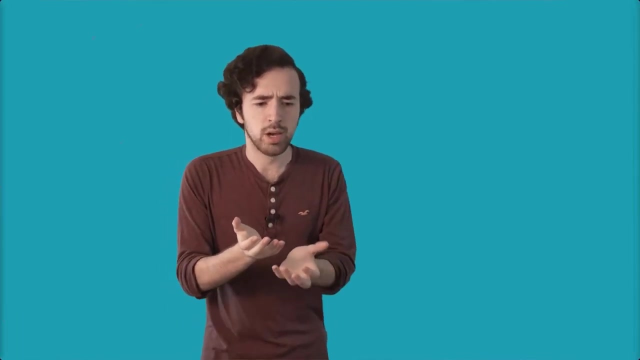 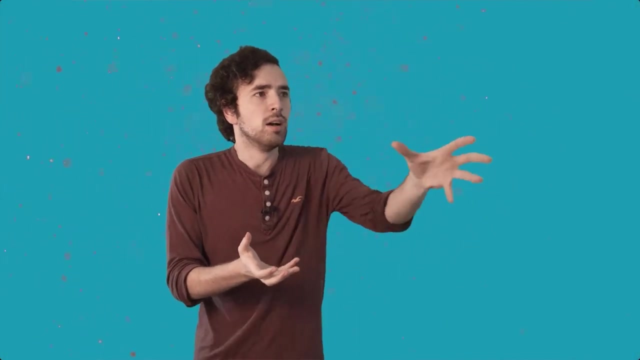 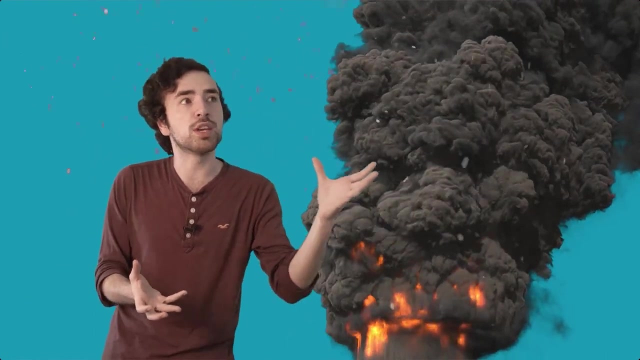 pancake into your mouth when you're suddenly interrupted by a booming rumble, The Earth beneath you begins to shake, Roof tiles begin to crack and fall all around you when, all of a sudden, to your horror in the distance, molten rock begins to spew from the top of Mount Vesuvius, along with a huge dark cloud. 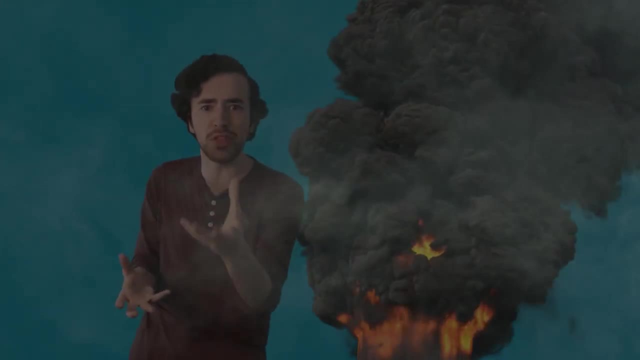 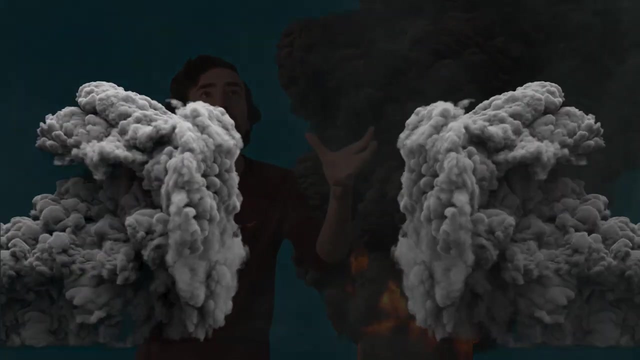 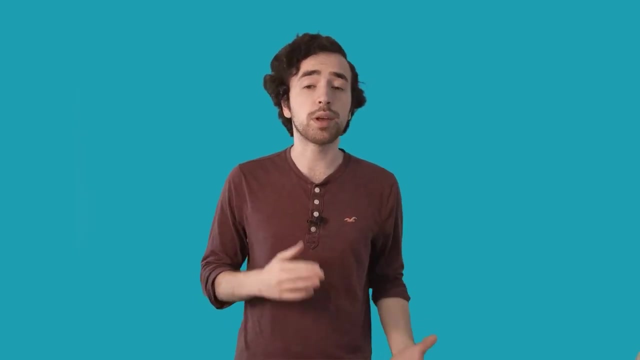 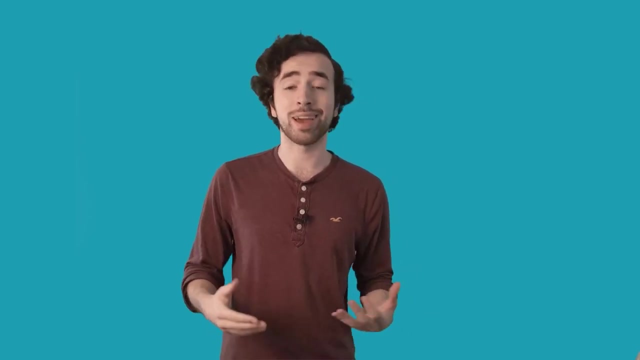 swallowing the city of Pompeii with it. You hear screams, confusion, and then darkness, as humongous blooms of ash blot out the sun. That is the exact scene witnessed and described by young Roman scholar, Pliny the Younger, whose uncle, Roman philosopher Pliny the Elder, died in what is perhaps the most infamous volcanic. 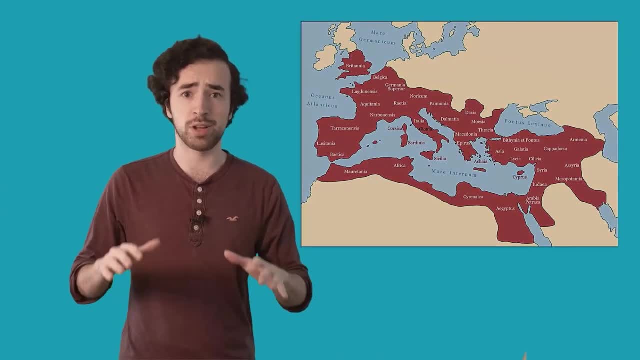 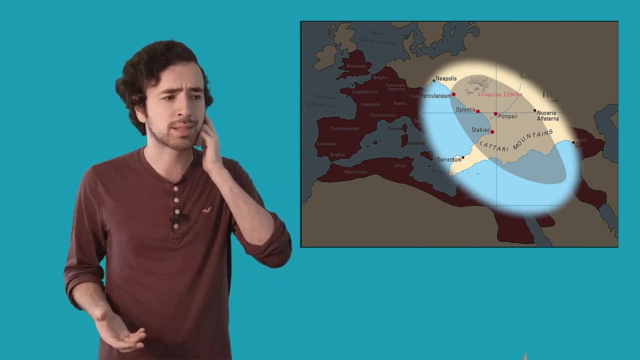 eruption in recorded history, The one that buried four Roman cities and killed two thousand people. Hold on. what was that? How did this happen? Good question. Volcanoes form when molten rock or magma breaks through the Earth's crust, The Earth's crust being. 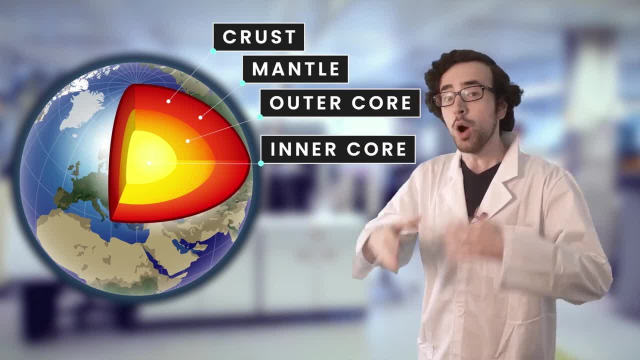 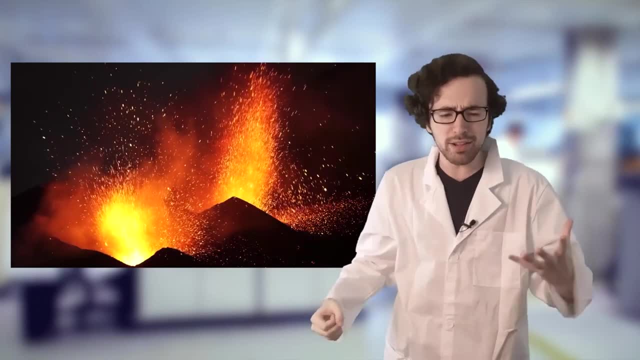 the top layer of the Earth covering the mantle, The mantle being the mineral layer covering the core. When magma with high pressurized gases breaks through to the surface, it erupts with enormous force, spewing rock, ash and lava for miles. 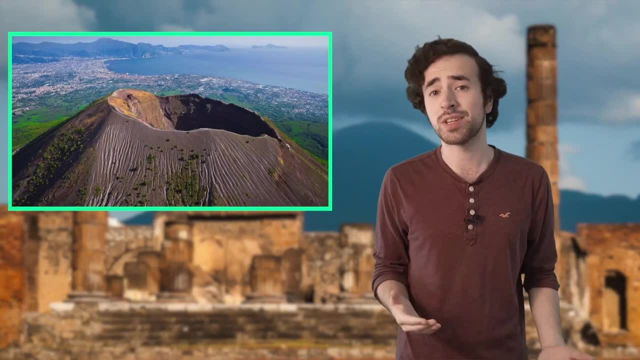 That is exactly what happened to Mount Vesuvius in 79 AD and the reason why Pompeii was buried underneath 30 feet of ash. That is exactly what happened to Mount Vesuvius in 79 AD and the reason why Pompeii was buried underneath 30 feet of ash. 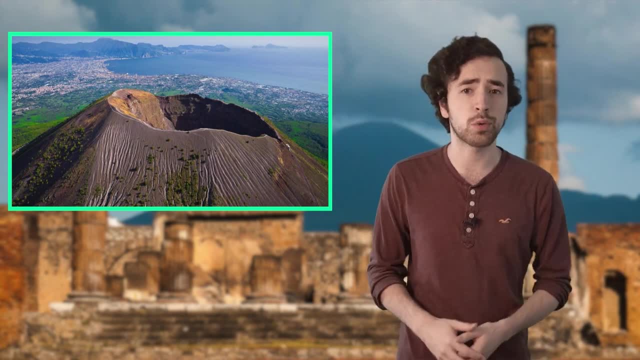 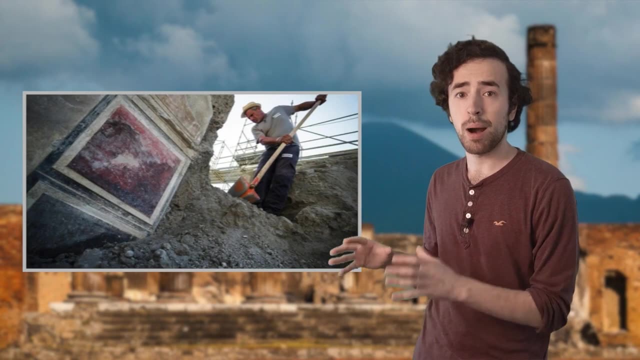 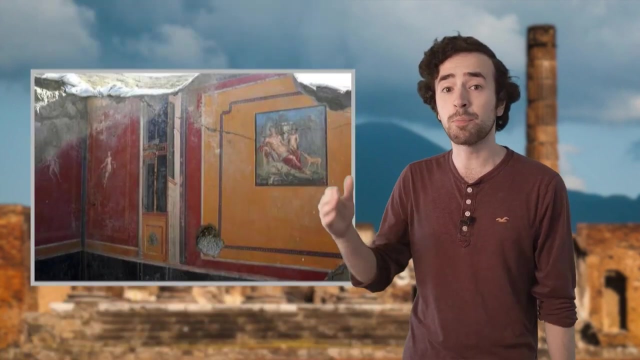 And remained buried underneath 30 feet of ash until 1748, when explorers digging there made an amazing discovery. Underneath all that ash, Pompeii was perfectly preserved, exactly as it was almost 1700 years ago. The people of Pompeii, and even the pets, like this guard dog here, were perfectly captured. 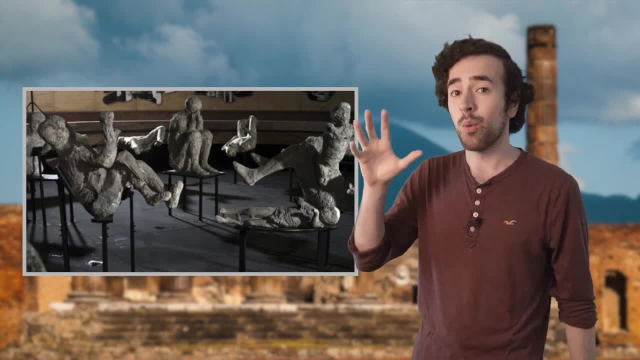 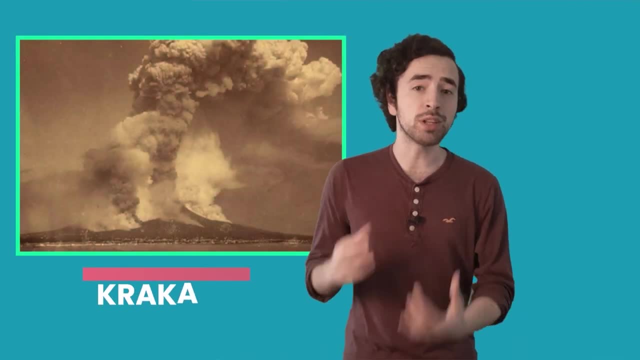 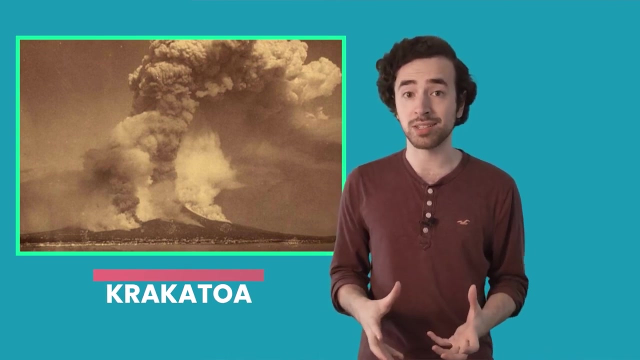 in the exact moment of what they were doing when that ash cloud swallowed them. Another infamous volcanic eruption was when Krakatoa in Indonesia erupted in 1883, throwing 5 cubic miles of Earth 50 miles into the air, causing temperatures to drop. 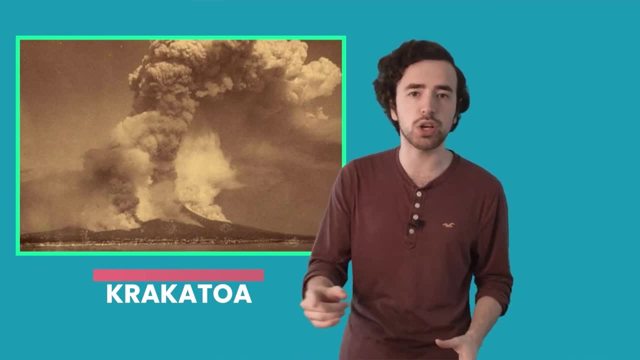 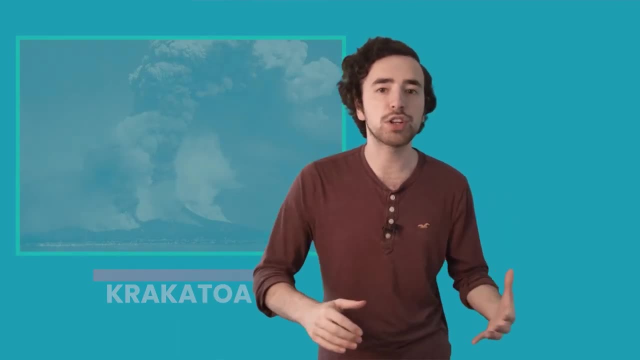 worldwide and creating a pressure wave that circled the globe three and a half times. The eruption was so violent that sounds of it could be heard on the island of Rodriguez, near Mauritius. The eruption was so violent that sounds of it could be heard on the island of Rodriguez, near Mauritius. 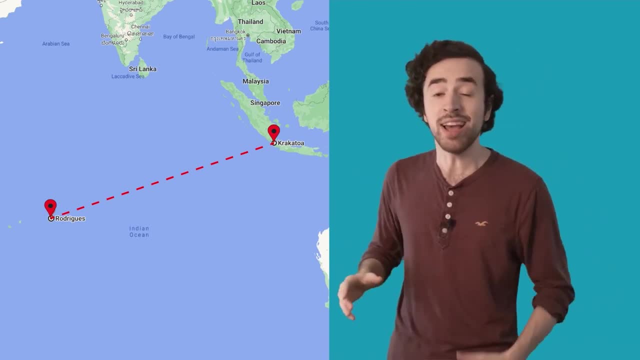 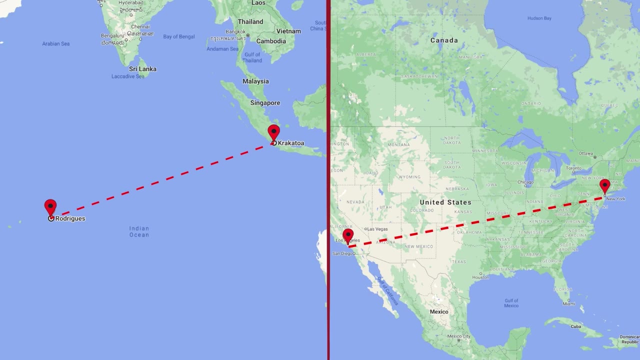 The eruption was so violent that sounds of it could be heard on the island of Rodriguez, near Mauritius, over 3000 miles away. That's further than the distance between Los Angeles and New York. Imagine for a second if something happened in Los Angeles and you heard it happen in New York. That's how powerful the Krakatoa eruption was. In terms of quantifiable energy, the force resulting from the eruption was equivalent to 200 megatons of TNT, That's 13,000 times the yield from the atomic bomb that devastated Hiroshima. 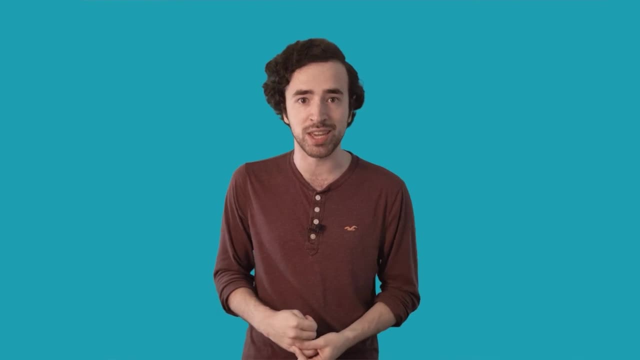 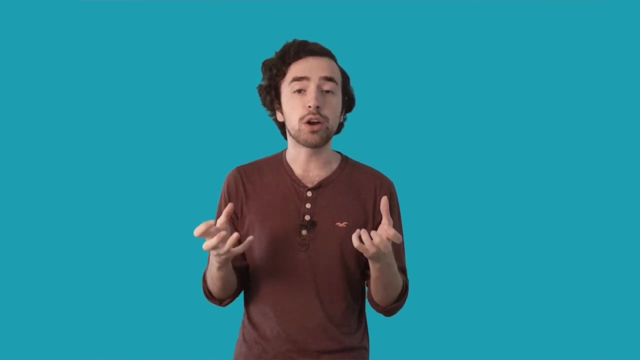 Japan and 4 times greater than the explosive yield of the largest nuclear device ever tested. We are talking about massive forces within the Earth capable of doing things like creating islands where there weren't islands before. capable of doing things like creating islands where there weren't islands before. 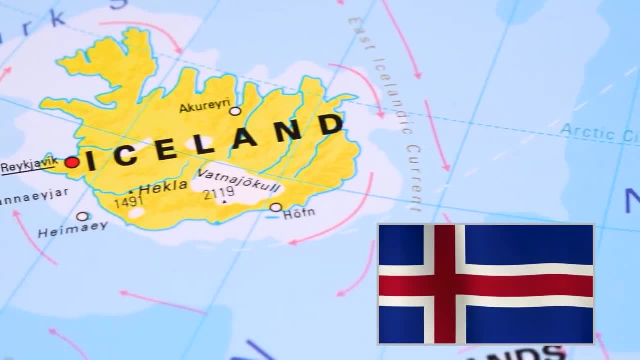 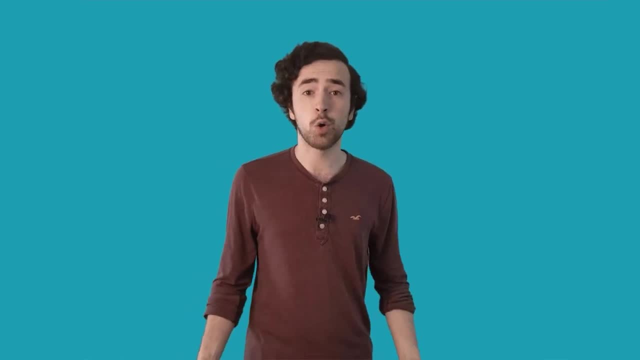 capable of doing things like creating islands where there weren't islands before, Islands like Iceland in the North Atlantic, one of the most volcanically active places in the world. Iceland is home to 130 volcanoes and the country has a population of only 357,000,. so that means one volcano for every 2,746 people. Tired of your hometown not having its own volcano, Consider relocating to Iceland One of Iceland's volcanoes named- Uh- how do you say that? Eyjafjallajökull. 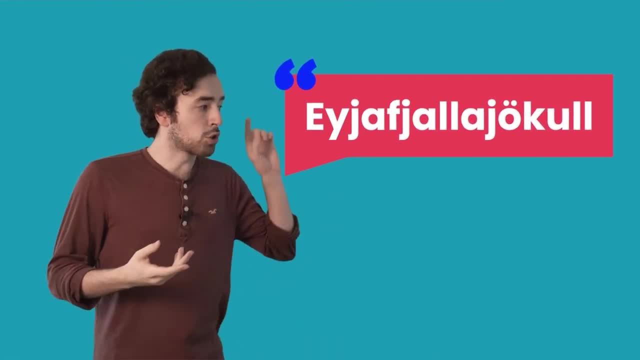 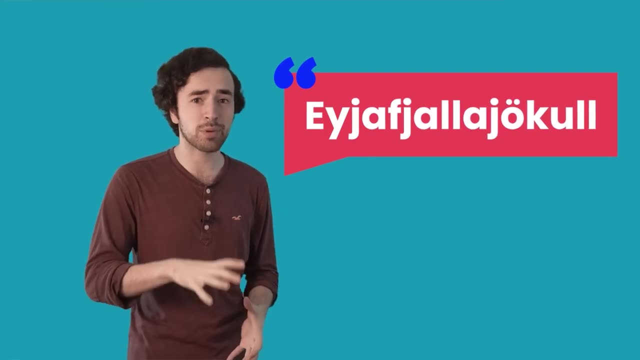 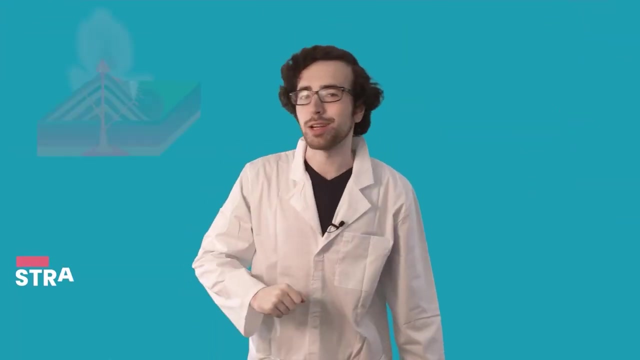 Oh right, of course, obviously. Um, so this volcano that starts with the letter E is a stratovolcano, completely covered by an ice cap. Hold on What? What's a stratovolcano, you ask? A stratovolcano is a volcano with thick, gummy limes. 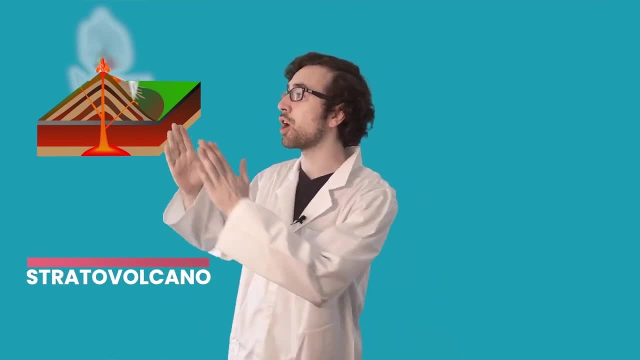 Lava that doesn't flow very far from where it erupted, meaning that the stratovolcano is taller and more conical, as opposed to a shield volcano, which is broader and many times wider than it is tall, because its lava isn't as thick and gummy. 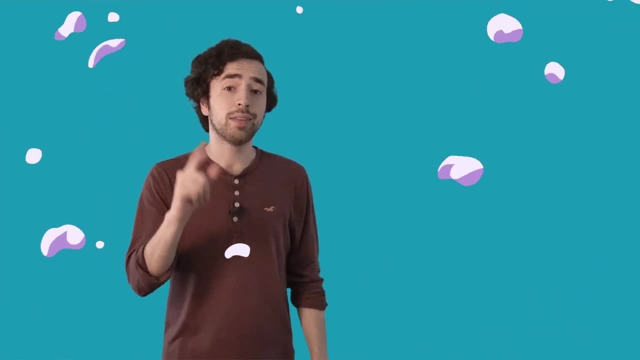 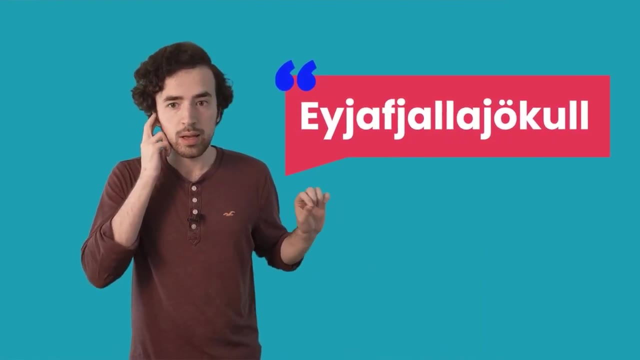 and therefore can flow further from the point of eruption. Anyway, this stratovolcano named- Okay, one more time, Eyjafjallajökull, Eyjafjallajökull, Nailed it- Erupted in April 2010.. 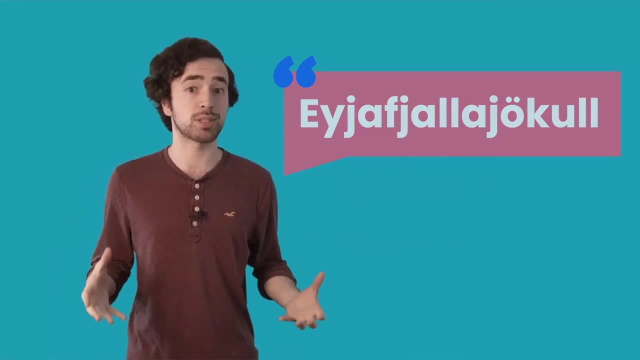 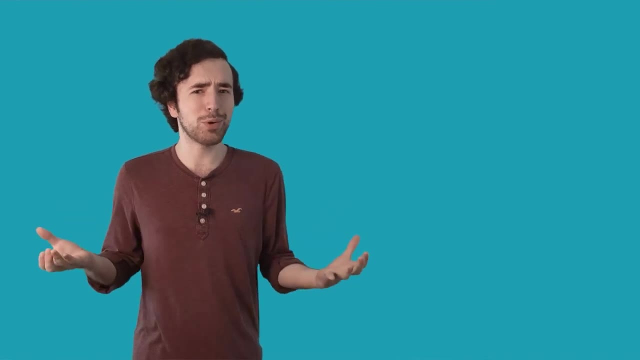 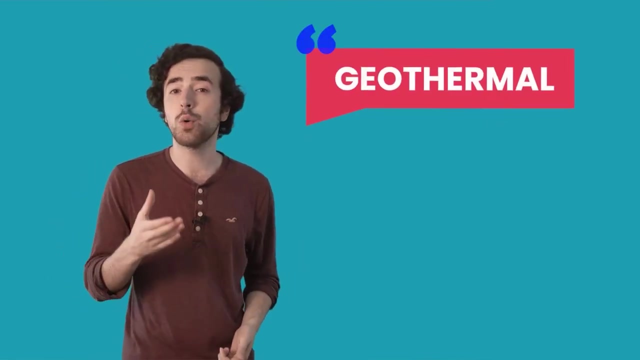 Darkening the skies with ash and causing massive, Massive disruptions to air travel all over Europe. So about now you're probably thinking: why on earth would anyone want to live near a volcano? Excellent question. One good reason to live near a volcano is to harness geothermal energy. 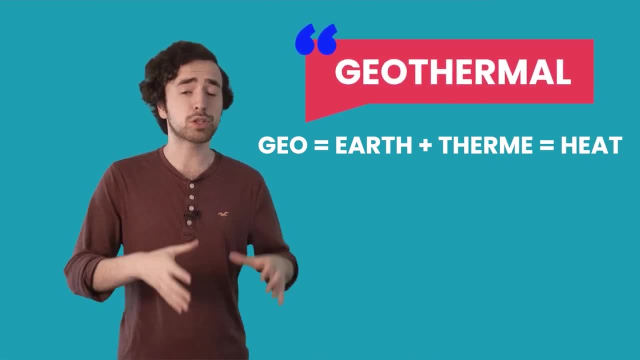 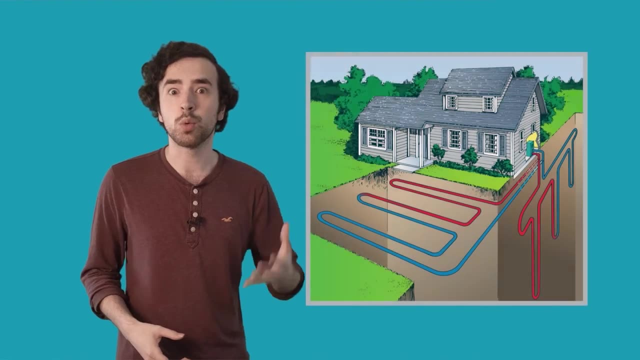 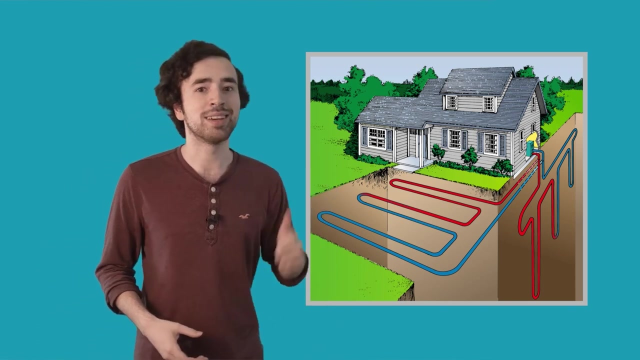 which is the heat from within the earth. Iceland makes great use of geothermal energy. As a matter of fact, 90% of Icelandic homes are heated with geothermal water, which is cooled and pumped straight from deep within the ground directly into taps. 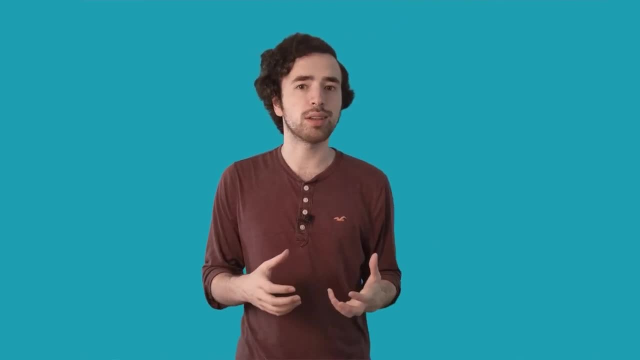 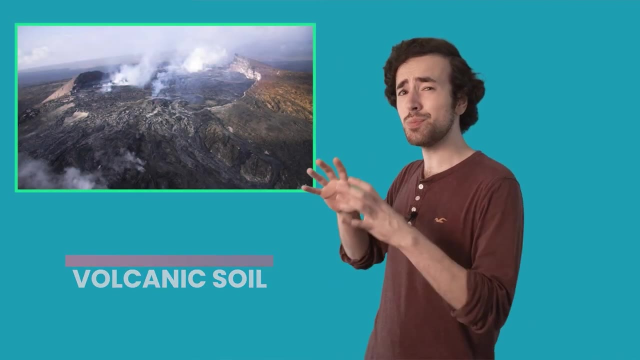 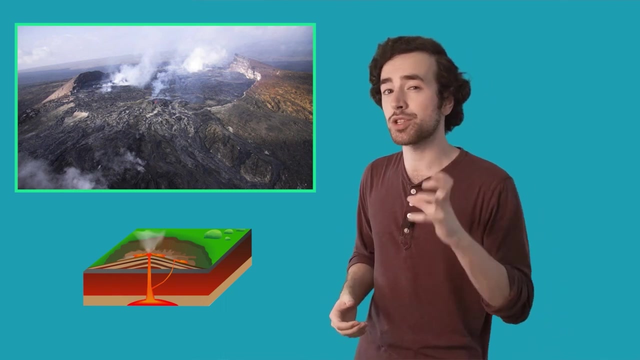 Another great reason to live near a volcano is for the rich quality of volcanic soil. Mauna Loa in Hawaii, which is the largest active volcano in the world and a superb example of a nice broad shield volcano, has been erupting on and off and depositing mineral-rich volcanic debris on the ground. 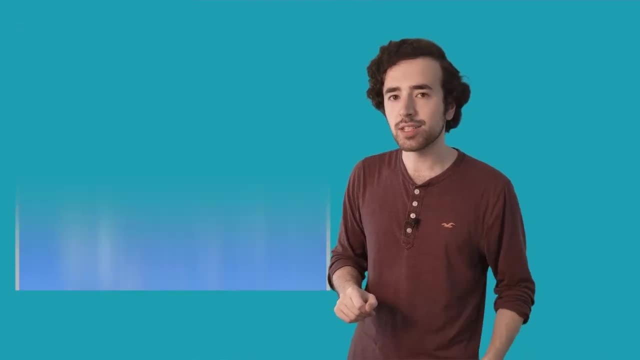 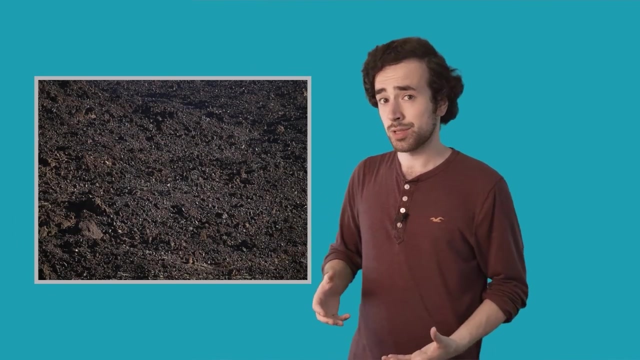 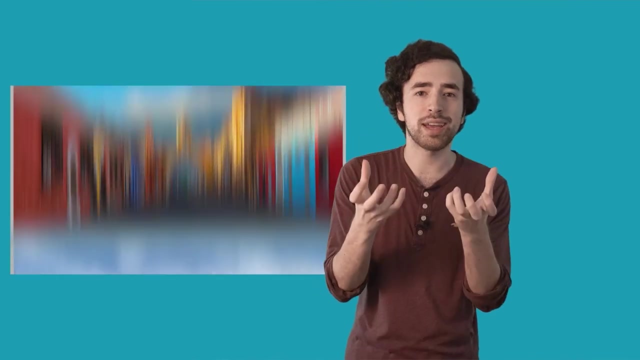 for the last 700,000 years. This volcanic debris gets weathered or broken down by rain and erosion over time. The result: Hawaii and other volcanically active areas like Antigua, Guatemala, have rich volcanic soil that can be used to grow a wide variety of plants. 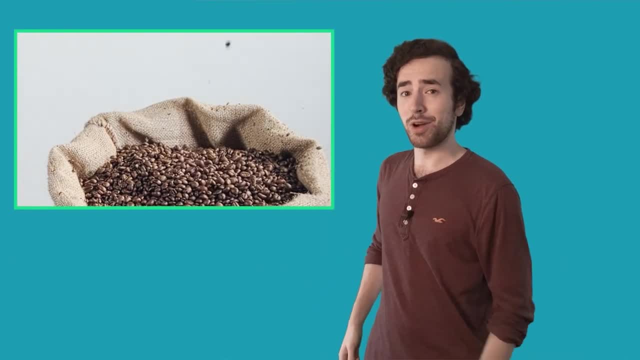 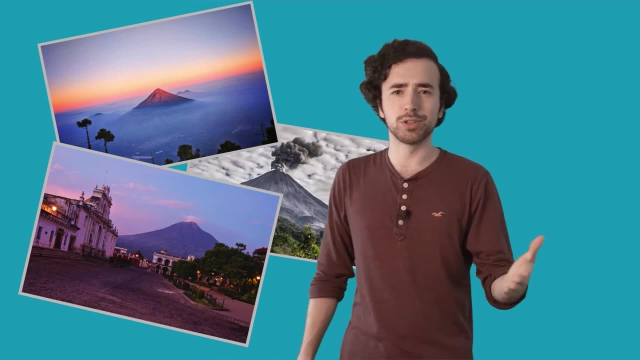 Plants like coffee. That's right, folks. If you want to grow world-class coffee in the shadow of not one but three stratovolcanoes, consider relocating to Antigua, Guatemala, where the coffee is three times as volcanically delicious. 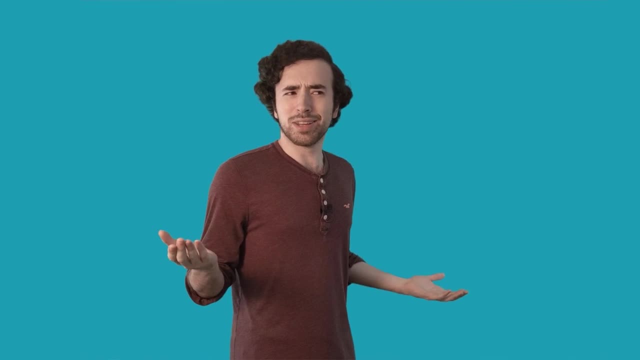 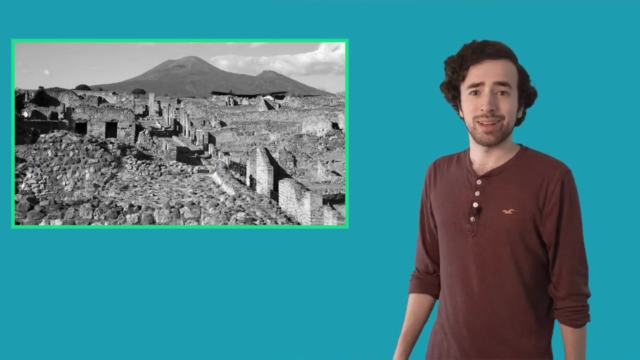 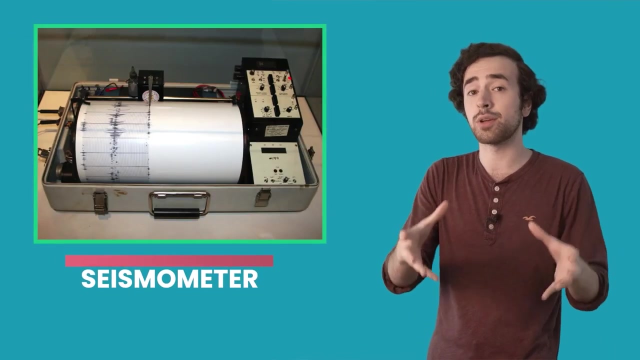 Now I bet you're thinking at this point: isn't living near an active volcano kind of dangerous? You bet it is. Look at what happened to Pompeii. That's why nowadays, geologists use technology like seismometers to record little earthquakes in the areas around volcanoes. 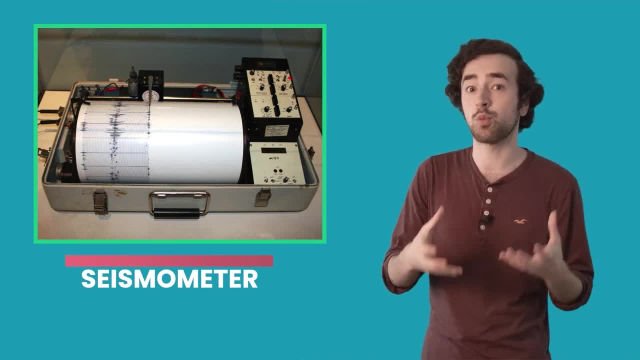 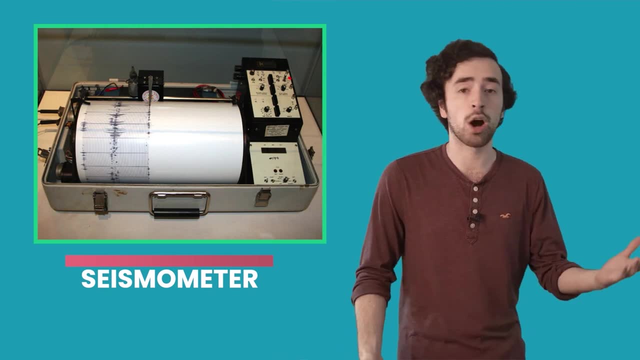 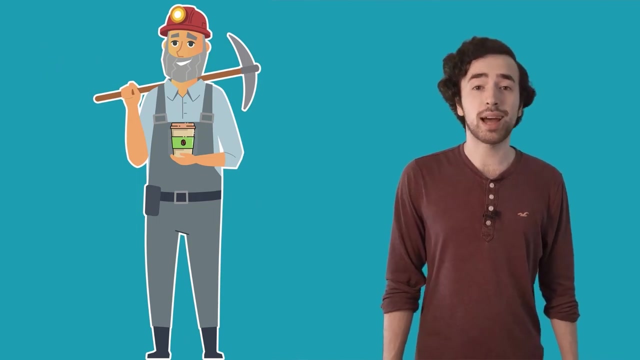 These earthquakes can be used to predict whether or not a full eruption can occur. So if you choose to relocate to an active volcano to grow your coffee, maybe consider sharing some of that coffee with your local geologists, because they're the ones keeping an eye on that volcano. 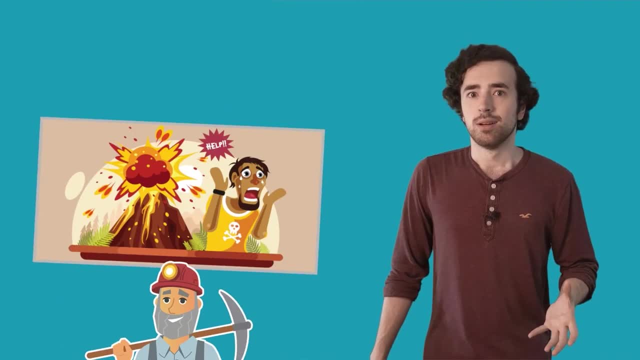 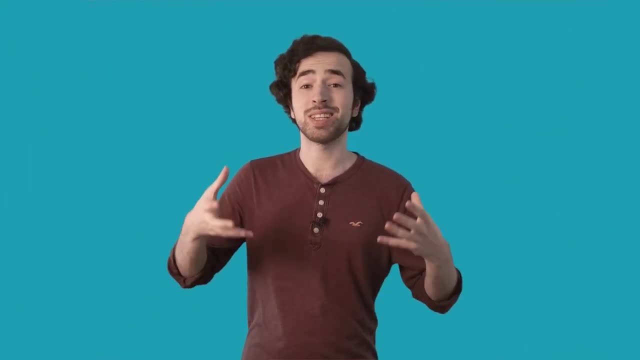 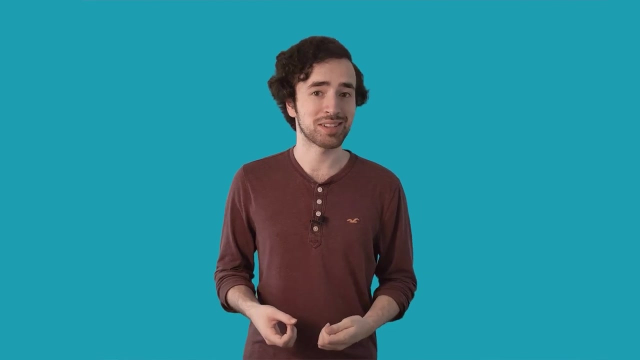 and gonna be telling you whether you should stay or run. Now I just mentioned earthquakes, which is another potentially catastrophic natural disaster that comes from the Earth. So how do earthquakes work? Glad you asked. The solid outer layer of the Earth called the lithosphere. 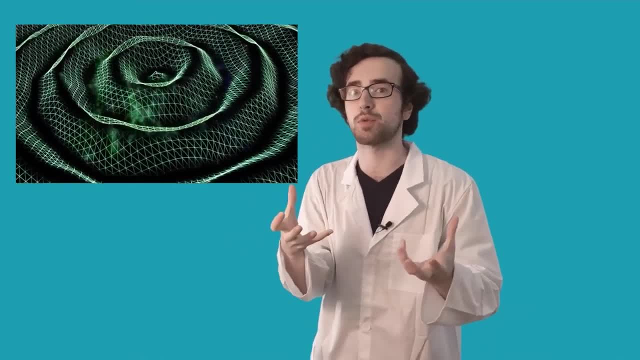 consists of the crust and the upper mantle. It splits into 15 to 20 huge slabs of rock called tectonic plates. Heat from within the Earth causes these tectonic plates to move and their edges stick together along points of friction. 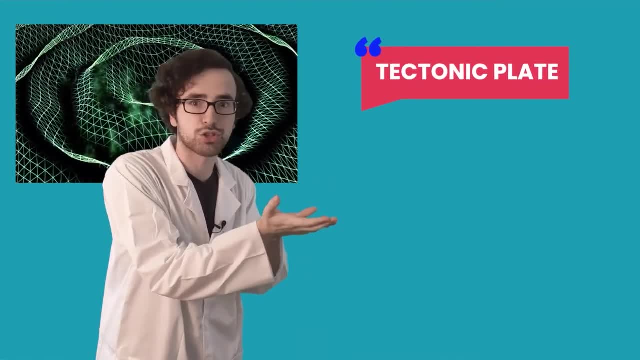 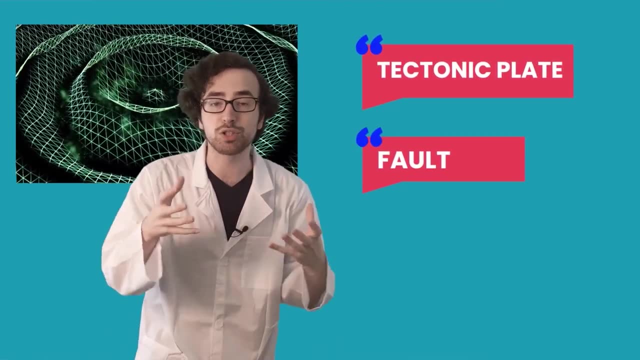 If a tectonic plate's motion overcomes this friction along a fracture zone or a fault that causes the shaking that we know as an earthquake, And if the same process happens underwater, that resulting earthquake could create a huge ocean wave, called a tsunami. 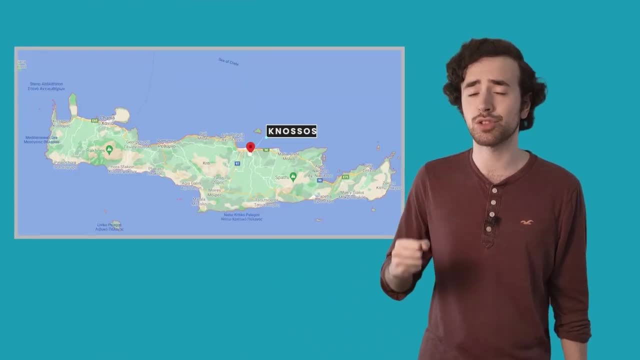 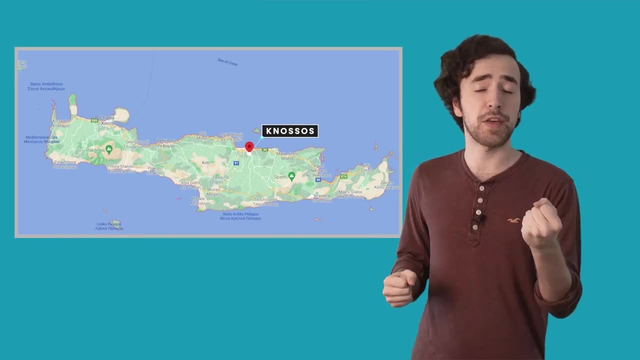 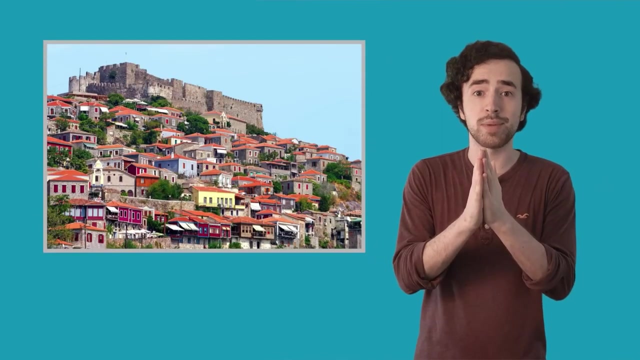 In 400 BC, a massive earthquake struck near Knossos, Crete, in conjunction with a massive volcanic eruption. that happened on the local Greek island of Thera, now called Santorini. The earthquake, the volcanic eruption and the resulting tsunami. 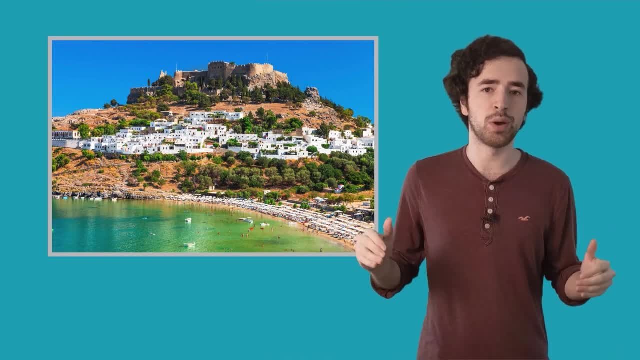 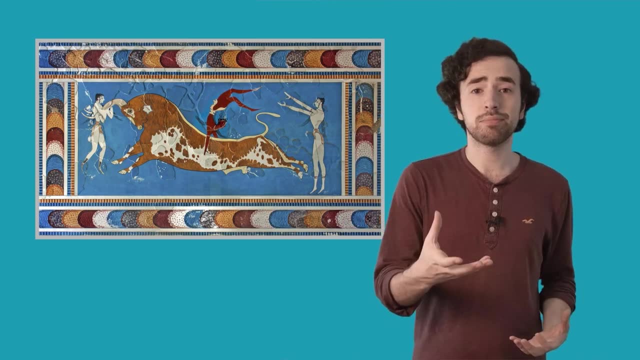 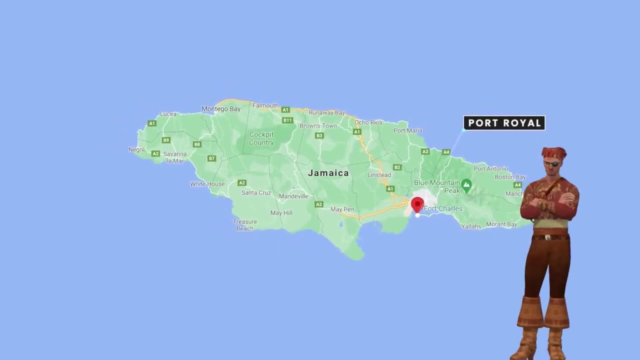 is credited with wiping out the entire Minoan civilization, a Bronze Age civilization that's renowned for its great cities, its writing and its works of art. Port Royal in Jamaica in the 17th century was a haven to all sorts of nefarious characters in the Golden Age of Piracy. 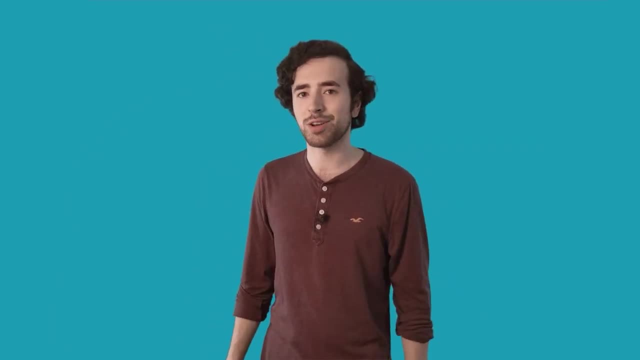 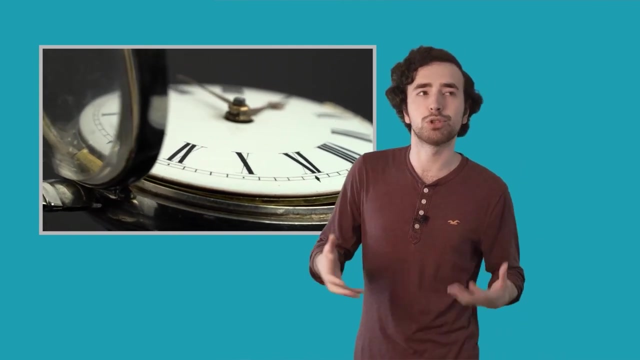 It, too, was also wiped out by an earthquake and resulting tsunami on June 7, 1692, at 1143 in the morning. How do we know that? Because a pocket watch stopped at 1143, was recovered some 270 years later.